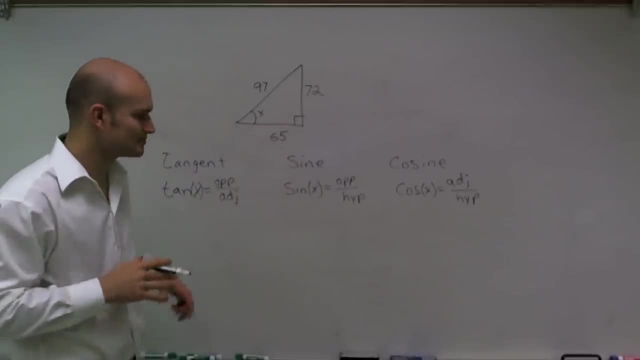 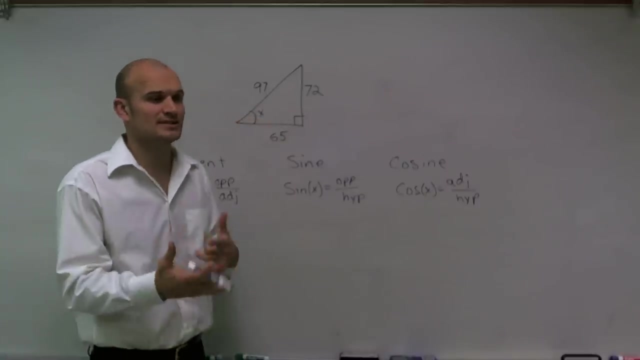 my right angle and also by using my x. So when I look at this and I see my angle x, one thing I need to determine is where the hypotenuse is And hopefully, if you guys work down the Pythagorean theorem, remember the hypotenuse is always your longest. 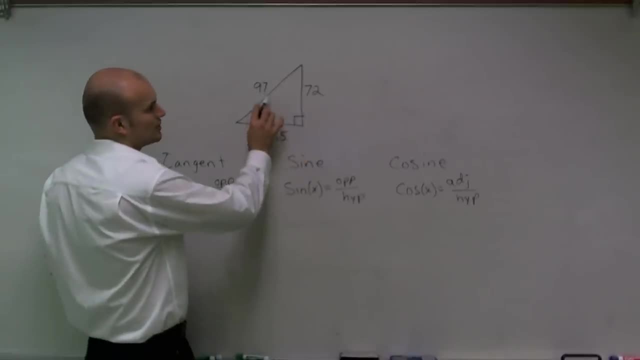 longest side of the triangle. It's also the side that's directly across from my hypotenuse, or directly across from my 90 degree angle, So we can label this side my hypotenuse always. Now, your opposite and your adjacents are always going to kind of change depending on which angle you have. So here's my 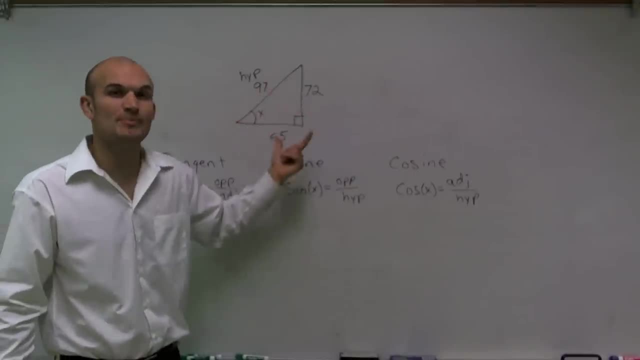 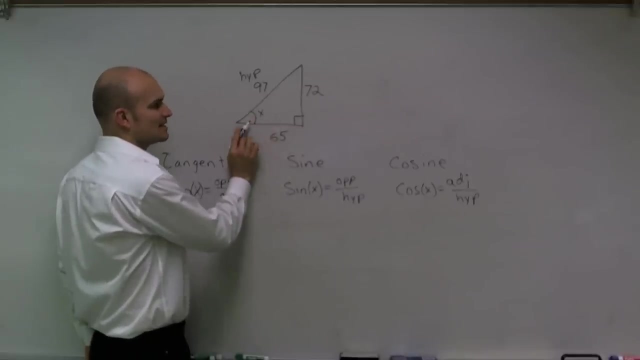 right angle, Depending on which angle I choose, is going to really depend on which one is my opposite, which one is my adjacent. So if I have this angle x, the side that's adjacent is going to be the side length that's going to connect your angle with your 90 degree angle. So therefore I can say that 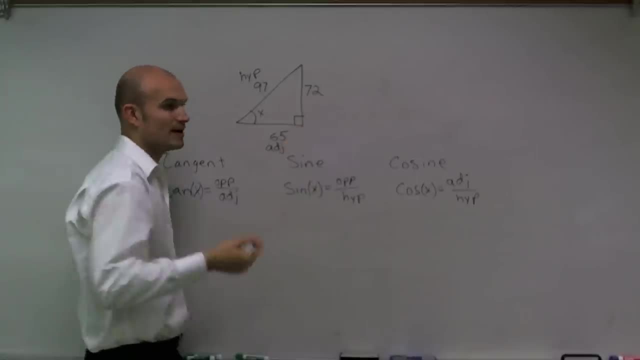 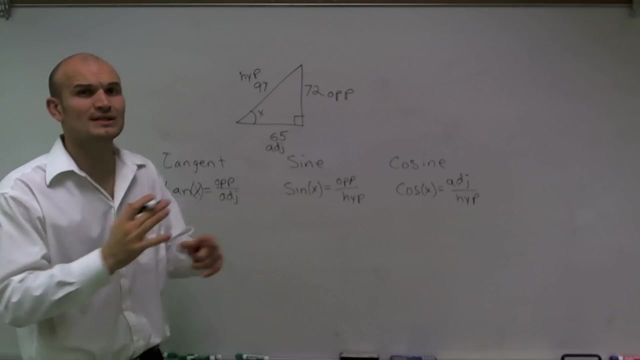 65 is going to be my adjacent side. Therefore, by process elimination or one way to always look at it is, your opposite is always the x side length that's always opposite of your original angle. So we can also say that 72 is going to be my opposite. Now for this problem, we only need to choose one. 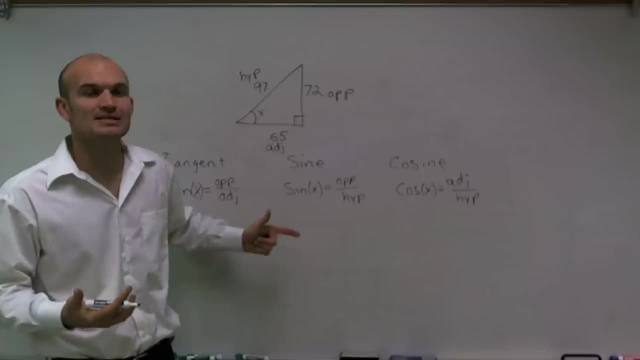 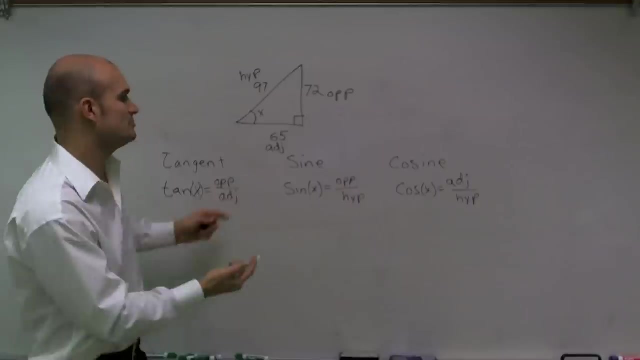 function that we'll work with. But since they gave us all three sides, I want to show you that it doesn't matter which function you choose. either one you pick, you're going to pick the right one, as long as you make sure you plug in the right one. So I'm going to plug in the right one and I'm 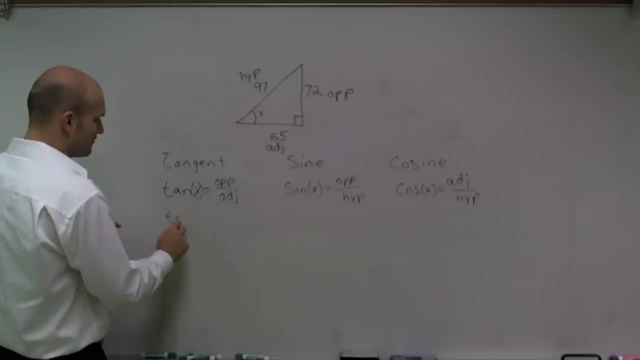 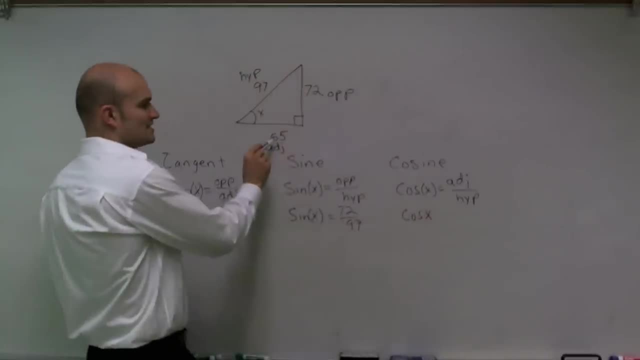 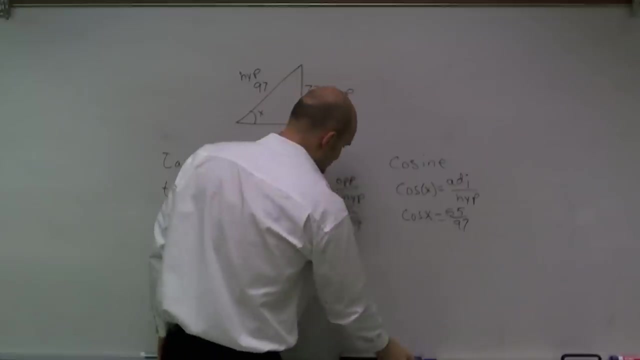 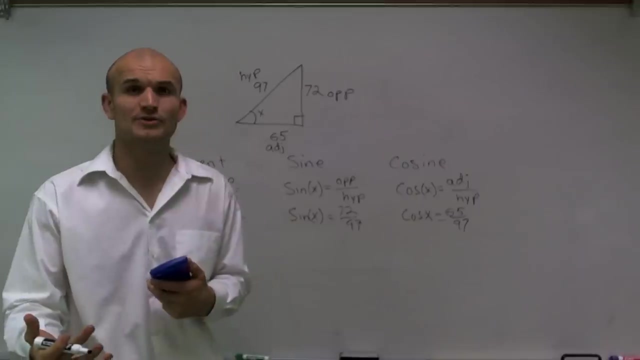 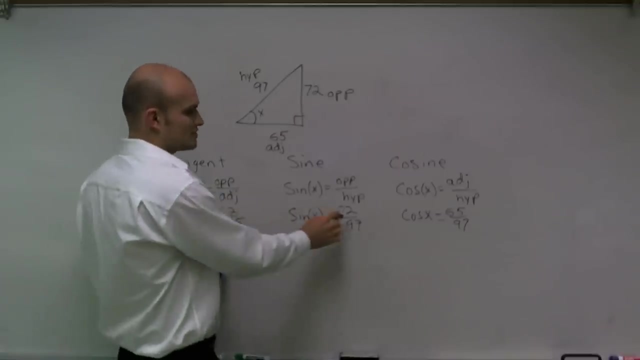 Sine of x is going to be the opposite, over my hypotenuse, which is 72 over 97. And therefore the cosine of x is my adjacent side, 65, over my hypotenuse 97.. Now it'll be helpful for us to look at some of the decimals for these problems. and when you're using the decimal, I want you to use the full decimal in your calculator. I don't want you to abbreviate, but I'm just going to write down a little bit of abbreviation decimal so you can understand that each one of these ratios are different. 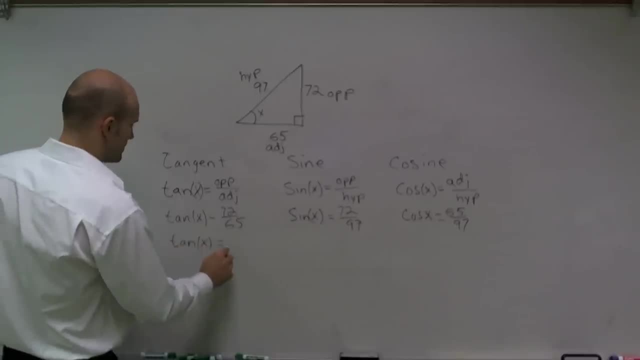 So the tangent of x is going to be, let's see, we'll have 72 divided by 65. And I'm just going to abbreviate this, like I said, 1.107.. Alright, the sine of x is going to equal 72 divided by 97,. 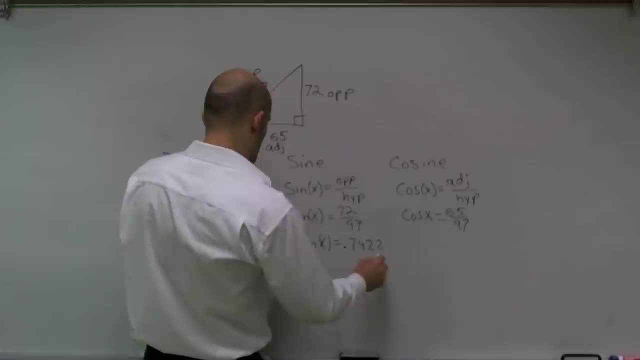 which is .74, 22,. and the cosine of x equals 65 divided by 97,, which is .6701.. Alright, so notice, my ratios are all going to be the same, But what I want to do, remember: we want to find the value of x. 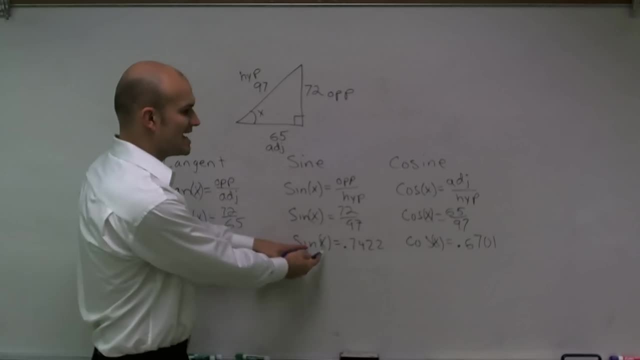 So right now we're taking the tangent of x and we get that We're taking the sine of x or we're taking the cosine of x. So if I want to find exactly what the value of x is, I need to undo. 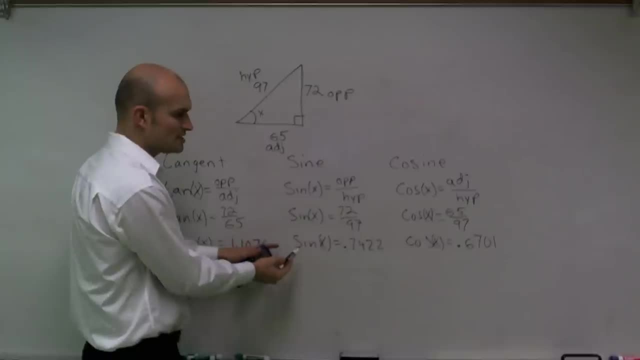 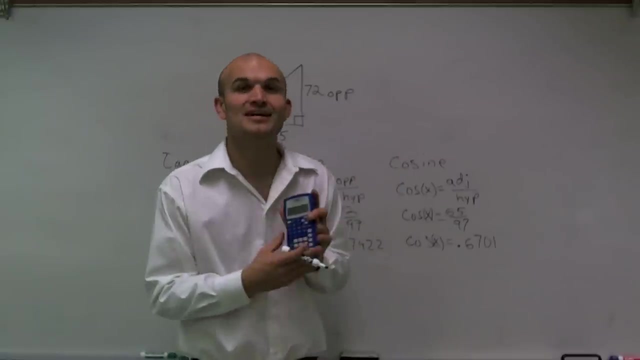 my functions. I need to undo the tangent function Undo the sine function, Undo the cosine function. So how do we undo those functions? Well, thankfully for our calculator, it's what we call the inverse function. So the inverse tan undoes tan. 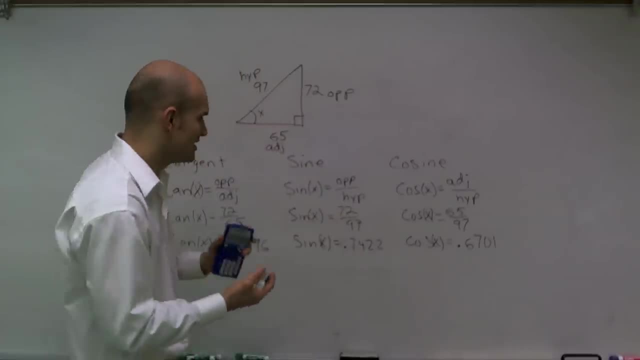 The inverse cosine is the inverse function of cosine And the inverse sine is the inverse function for sine. So what I'll write is: so if I take the inverse tan of what my value is, I'm going to get my angle. Now, like I said, I want to make sure that you guys put them in correctly. 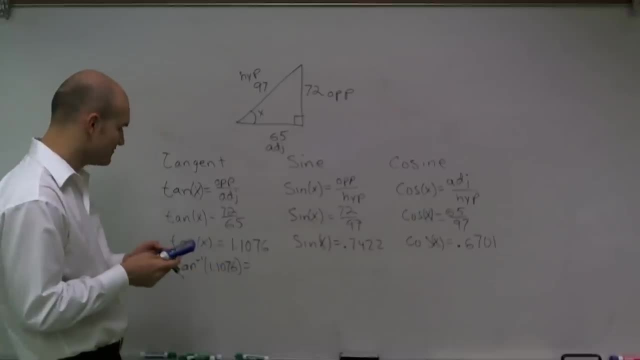 because I really do not want you to abbreviate. So I'm going to do 72 divided by 65. And then I'm going to take the inverse tangent of that answer And what I get is 47.9.. And I'm going to round that to 48 degrees.